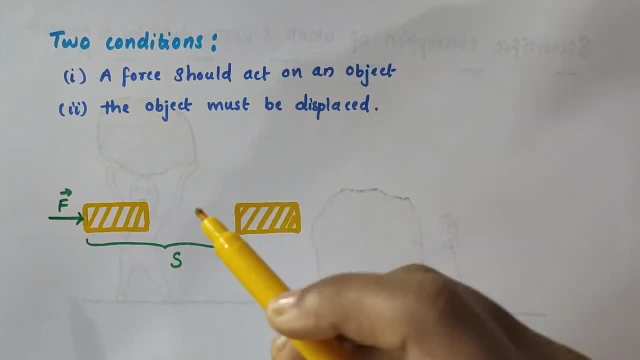 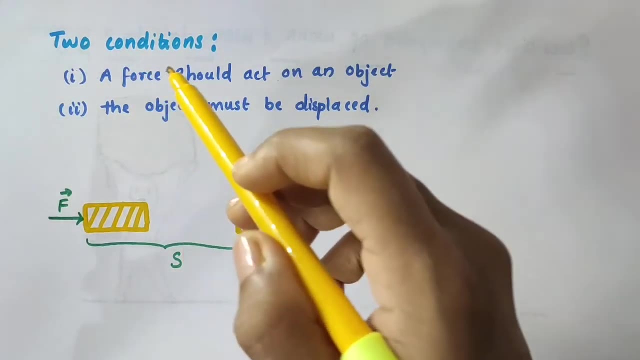 There are two conditions needs to be. I mean, there are two conditions need to be satisfied for work to be done. The first one is a force should act on- Okay, Okay, Okay, Okay. And the second one: the object must be displaced. 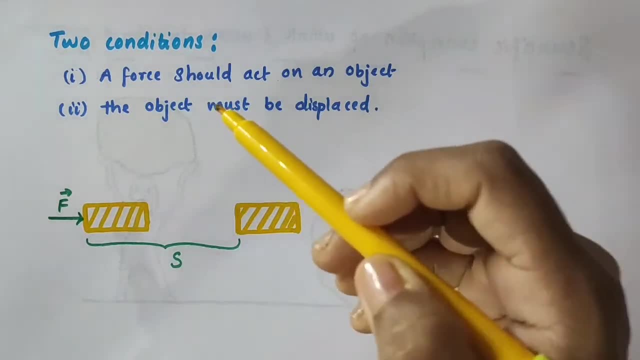 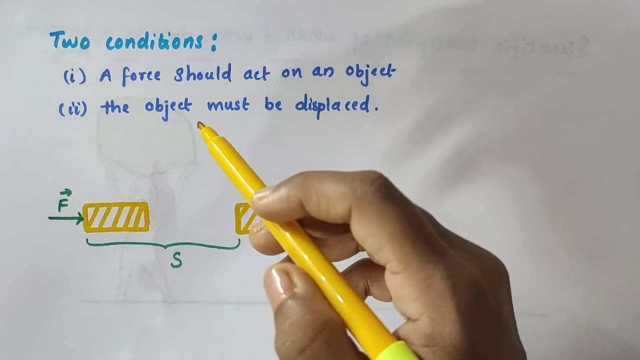 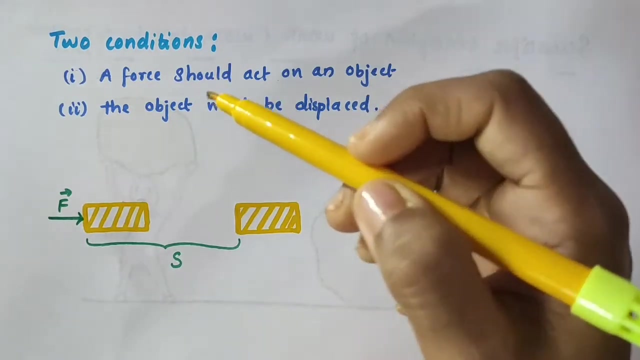 So there are two conditions need to be satisfied for work to be done. The first one is a force should act on an object, and the second one is the object must be displaced. If any one of these two conditions does not, I mean, exist, then work is not done. 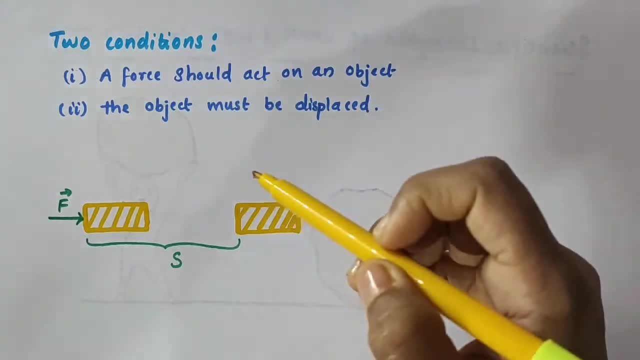 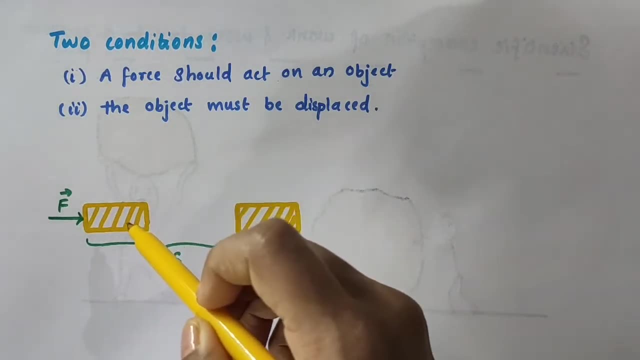 This is the way we view work in science. Now, how do we know that work is not done? How can we define the term work in science? Consider an object here. Let a constant force F act on this object along this particular direction, that is, to the right. 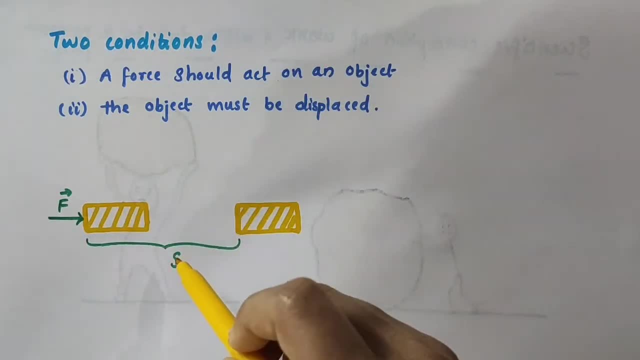 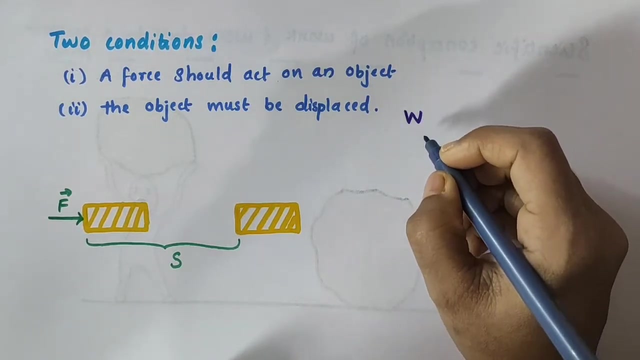 Let the object be displaced through a distance S due to the application of this force in the direction of force, that is, the object displaces to the right Right. Let W? W be the work done. We define work as the product of force and displacement. 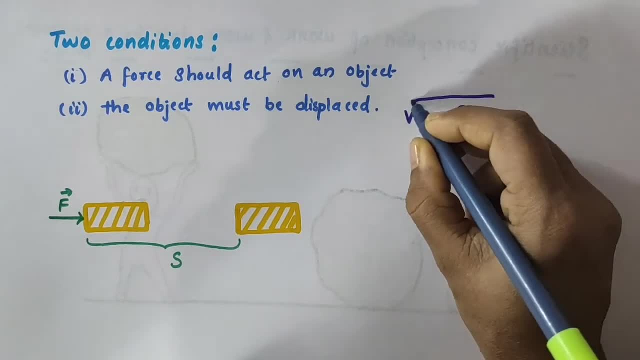 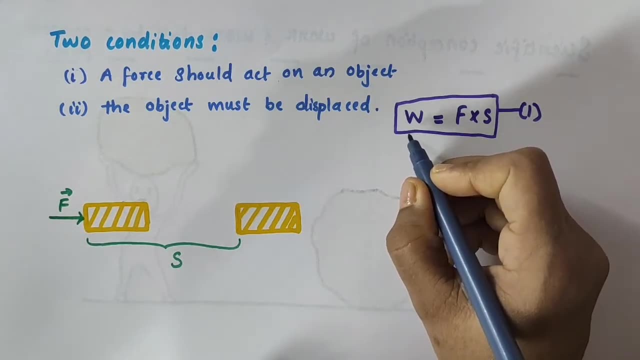 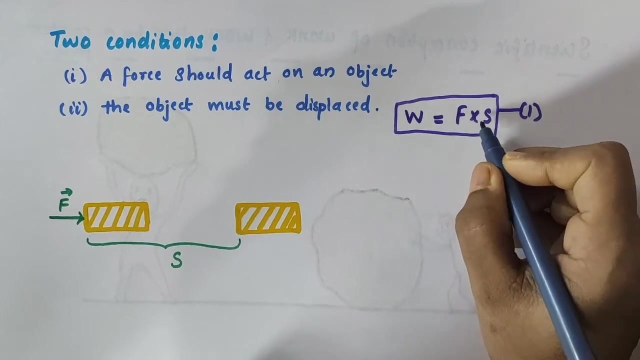 That is, W is equal to F into S, And I am taking this as equation number 1.. That is work done by a force. F acting on an object is equal to the product of magnitude of the force and the distance moved by the object. 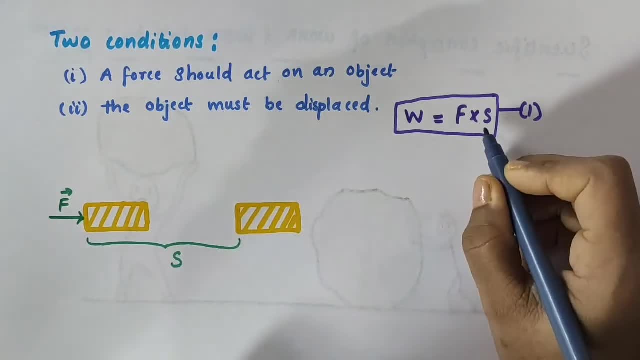 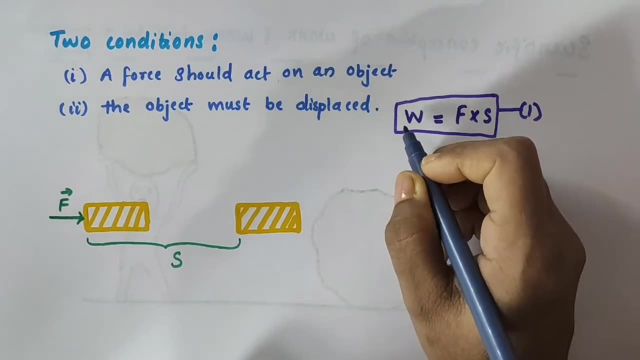 Okay, In the direction of force. In the direction of force or the displacement of the object? S Okay, Displacement of the object is S. Work is actually a scalar quantity, That is, it has only a magnitude. I mean, it has only magnitude. 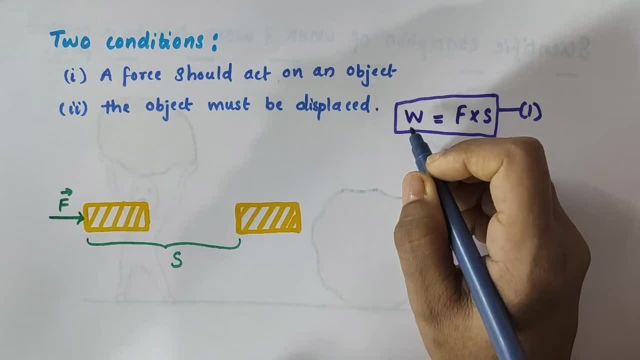 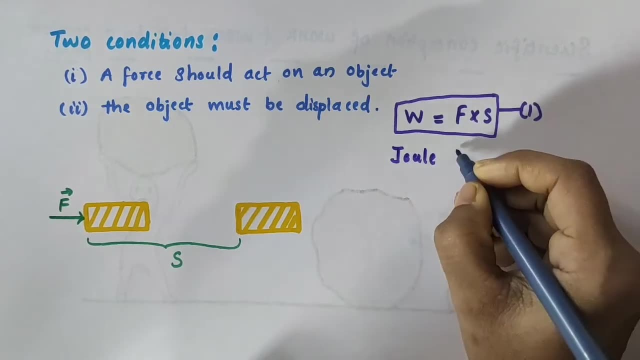 It doesn't have direction. Okay, It has no direction, Alright. So work is a scalar quantity. SI unit of work is joule And it is represented by the letter cap, letter J. So here I am writing the SI unit of work as joule. 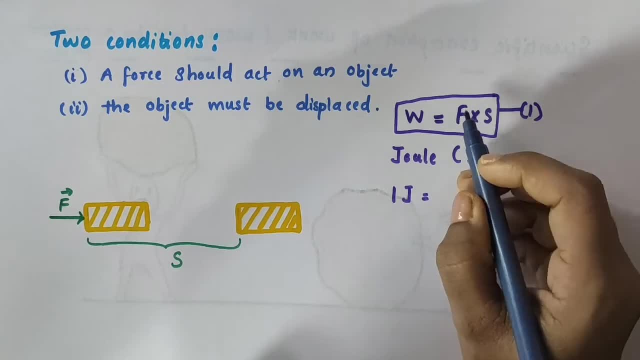 I am simply writing it as 1 joule. 1 joule is equal to What is the SI unit of force, Newton. So I am writing it as 1 newton Into SI. unit of displacement is meter. 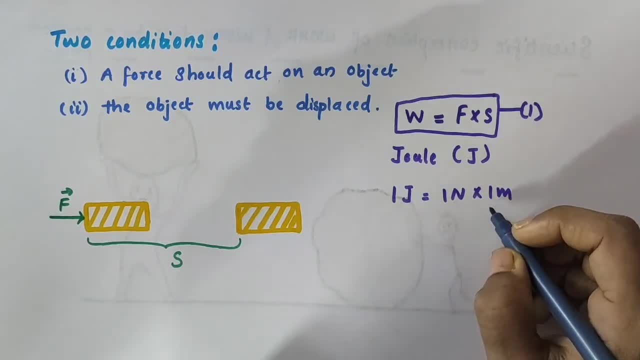 So I am writing it as 1 meter. Okay, That is, 1 joule is equal to 1 newton into 1 meter, Or joule is equal to newton meter. So SI unit of work is joule or newton meter. 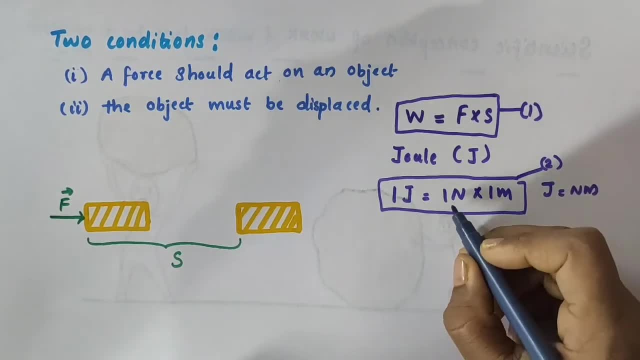 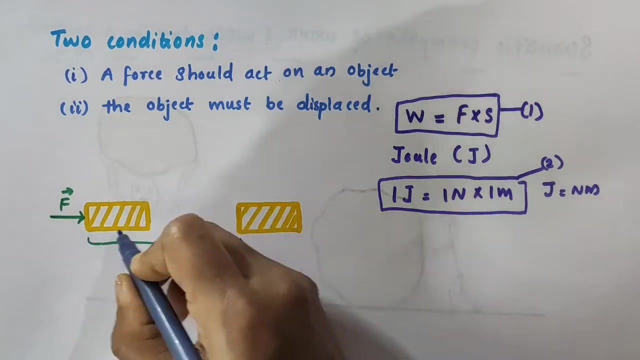 I am taking this as equation number 2.. Then from equation number 2. So we can say that 1 joule is the amount of work done on an object When a force of 1 newton displaces the object by 1 meter along the line of action of force. 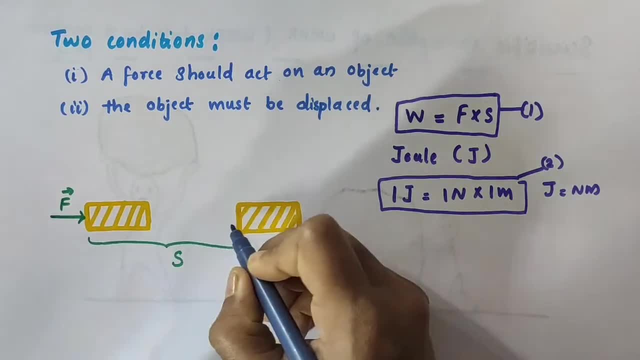 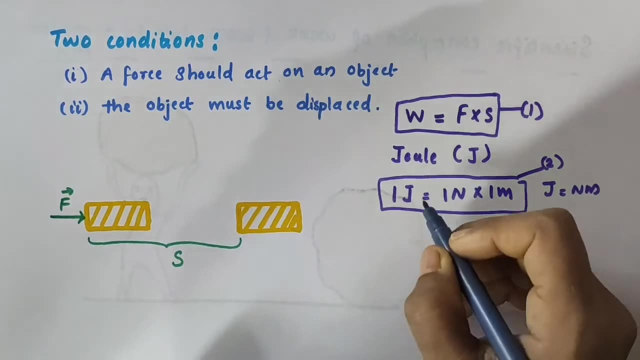 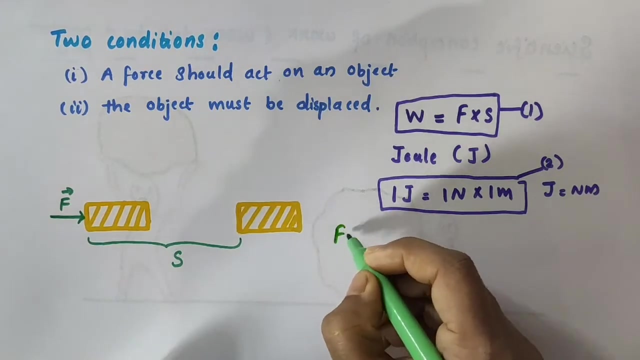 Okay, The force has exerted in this particular direction, towards the right, And the object has also moved along the same direction of force. Okay, Now if the force on an object is 0.. That is, if F is equal to 0.. 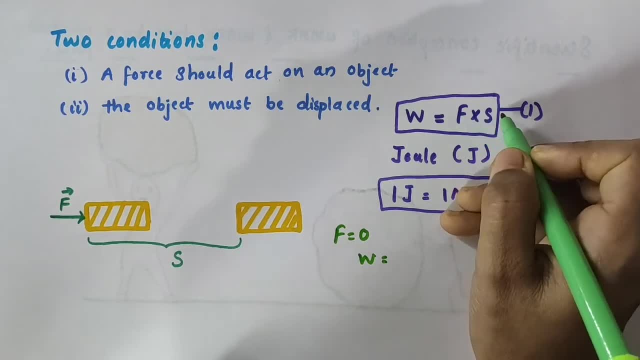 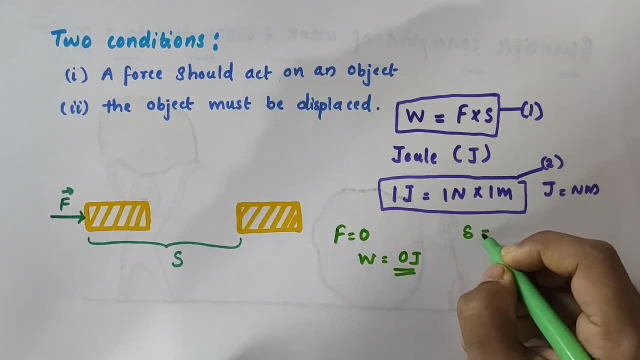 Then work done would be what W is equal to 0 into S. 0 into any value will give you 0. So work done would be 0 here. Similarly, if the displacement of the object is 0. That is, if S is equal to 0.. 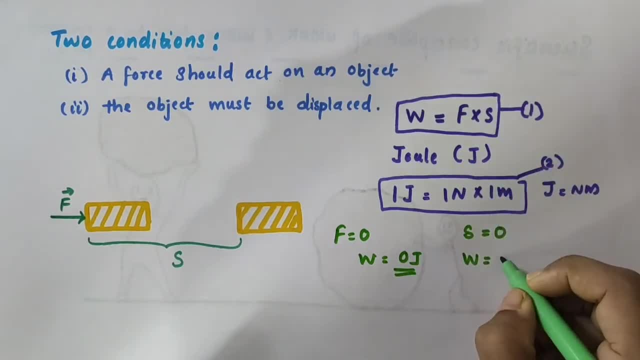 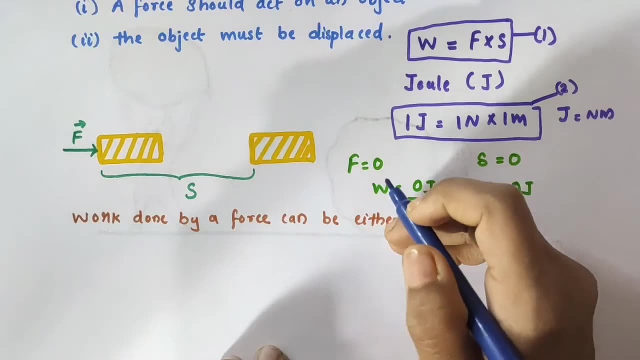 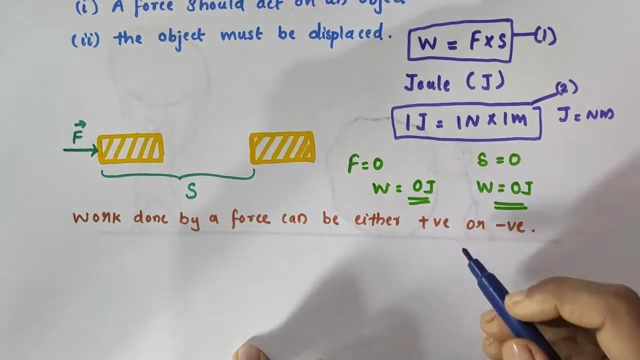 Then also the work done would be F into 0.. 0 into any value will give you 0. So work done would be 0.. Now you see, The work done by a force can be either positive or negative. Work done can be sometimes positive and sometimes it will be negative. 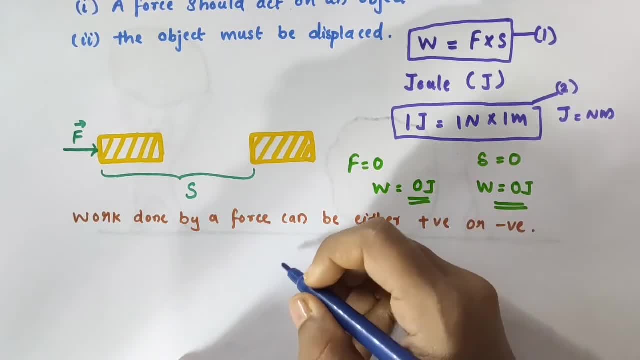 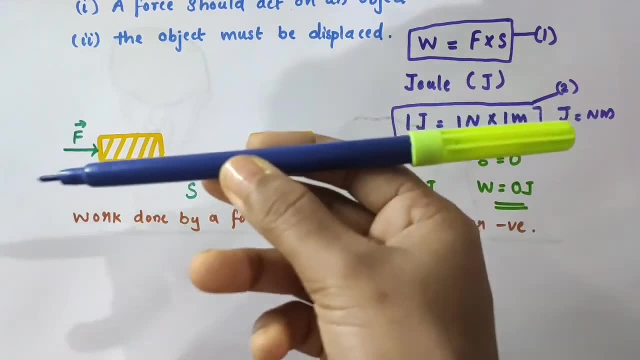 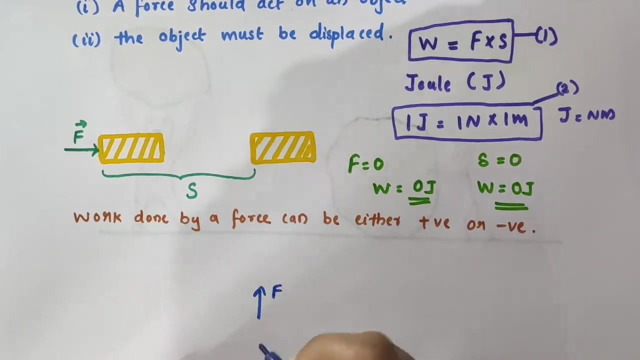 To understand this, let us discuss an example. When we lift an object, For example when we lift this pen, We exert a force on it in the upward direction. Okay, So we exert a force on this object in the upward direction. 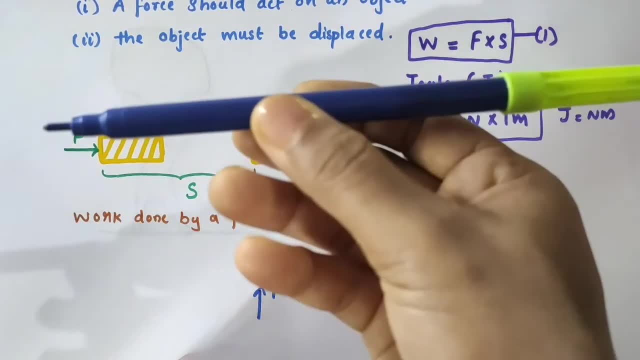 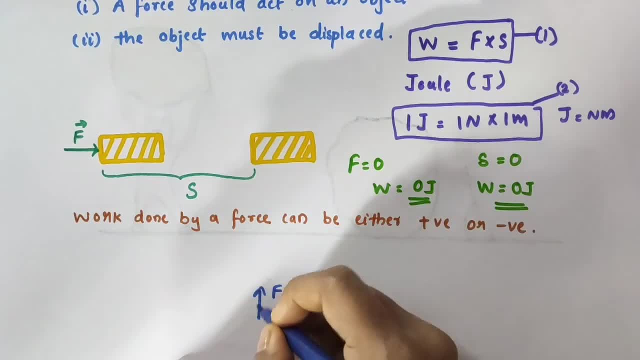 We exert a force in the upward direction. So we exert a force in the upward direction And the object also displaces in the upward direction. Okay, Object also displaces in the upward direction, Alright, That is In this case.